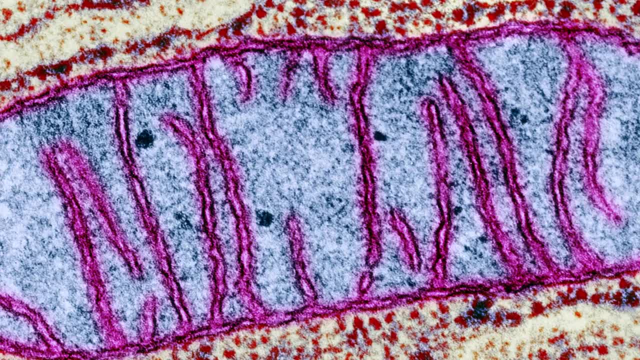 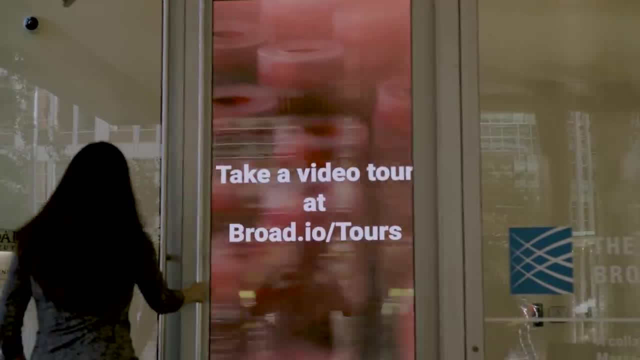 got me hooked. seeing the power of being able to accelerate the biology was really enticing to me. I run a research lab here at the Broad Institute of Harvard and MIT and what's really unusual about it is that we bring together a wide range of researchers and researchers from all over the 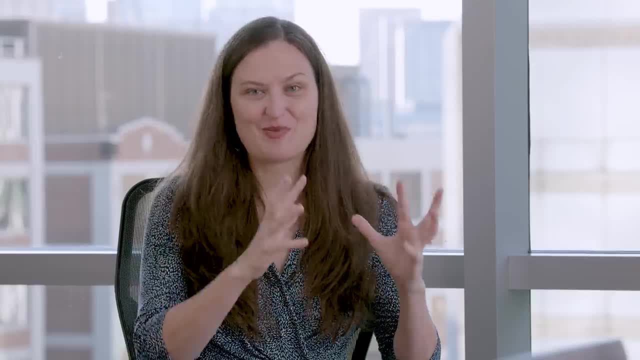 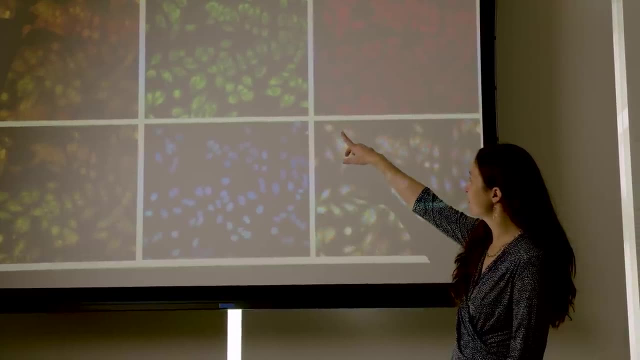 world. We bring together people at the interface of two disciplines, So normally there's biologists and there's computer scientists and we are right in between those two. It's a really cool place to be because it's uncharted territory and the synergy of everyone coming together with their 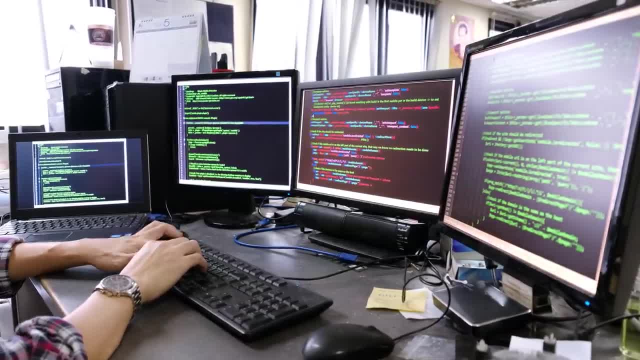 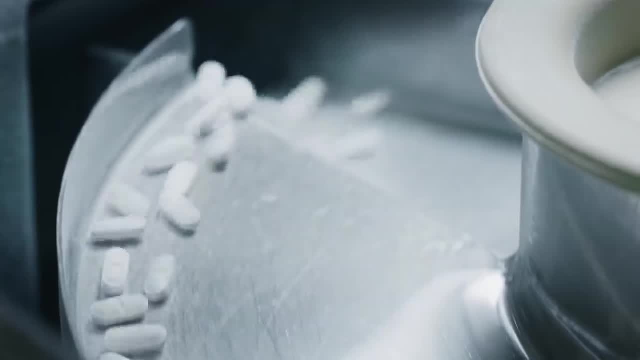 different ideas from different disciplines really helps to accelerate our research. So I got into this field because I wanted to develop new medicines. and it's an increasingly important problem as it's getting more and more expensive to find new medicines. and, on top of that, humanity is finding a way to develop new medicines. and it's an increasingly important problem as it's getting more and more expensive to find new medicines. and on top of that, humanity is finding 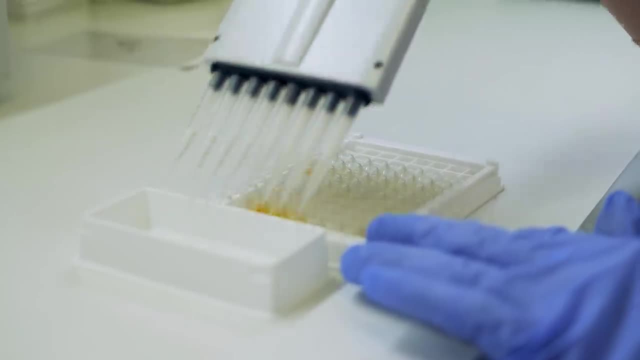 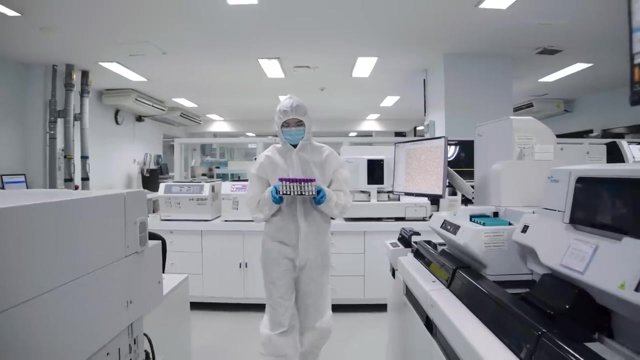 more and more diseases that we need to cure. The standard way of identifying drugs is that you just study a disease for a couple of decades, try to figure out the mechanisms. There's so much that's unknown and it's just incredibly painstaking. There's still a huge bottleneck in finding 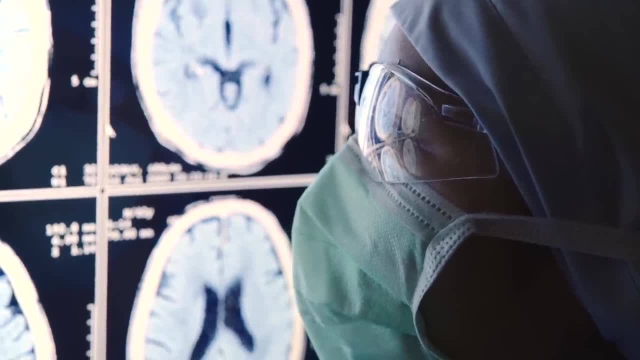 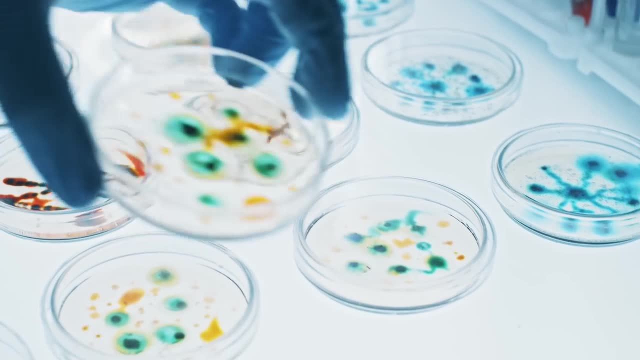 medicines for each disease, Instead of trying to study diseases in actual humans or even in model systems like a mouse or a rat. what if we could study the disorders in cells growing in a dish? They're super cheap, very easy to grow, but they're also very expensive to find and they're 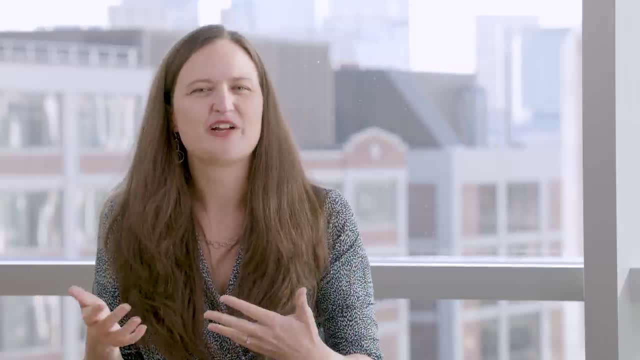 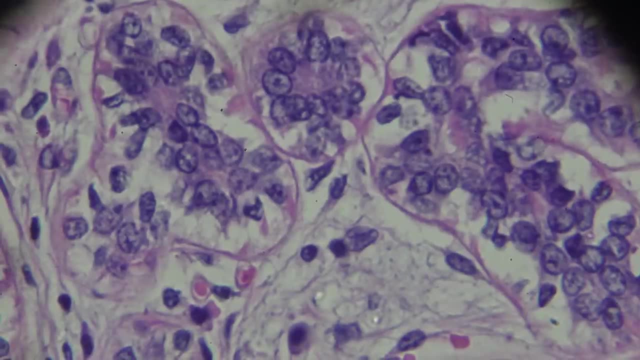 super cheap, very easy to find, and they're super cheap, very easy to find, and they don't mind if you add thousands of chemicals to them to try to figure out if one of them might make a good drug. So the approach that my lab is taking involves images. So we use microscopy, we use image. 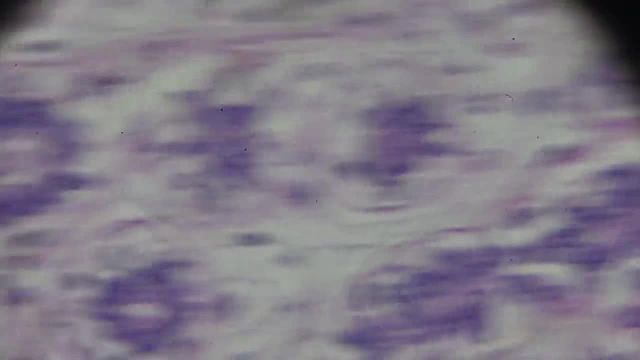 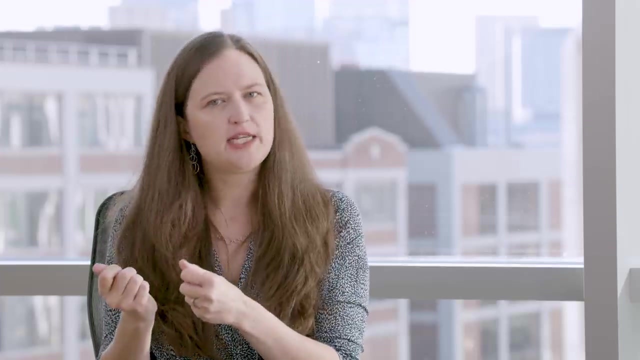 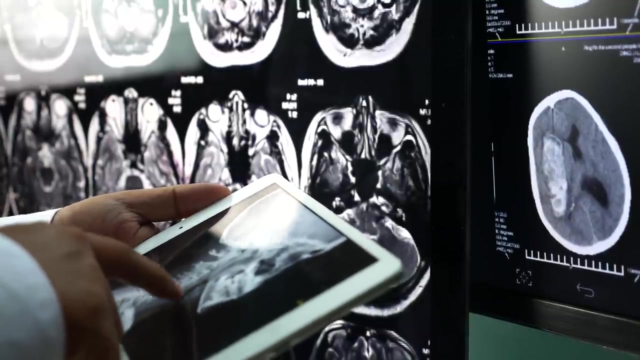 analysis to see whether we can identify any unusual structures in the cells of humans that have particular disorders. We can treat those cells with different drugs and try to find are there any drugs that make the unhealthy looking cells look healthy again. One example of this basic approach is what we've done with patients who have a lot of cancer. We've